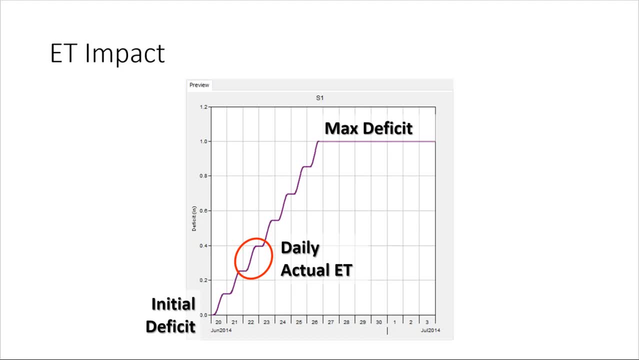 deficit increases when plant uptake draws water from soil storage. If no method for increasing deficit is specified, soil storage will fill up and infiltration will only occur at the specified constant rate. Here is an example of the impact of modeling ET on the soil moisture deficit. 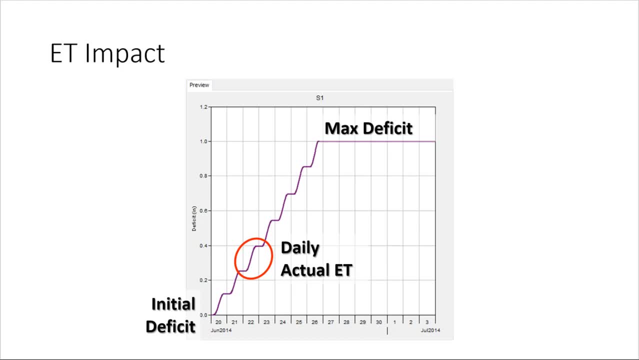 The initial deficit is zero. No water is input to this system. The diurnal cycle of ET creates a stair-step shaped accumulation of deficit until the maximum deficit is reached. The steepness of the growth is controlled by atmospheric conditions and the crop coefficient. 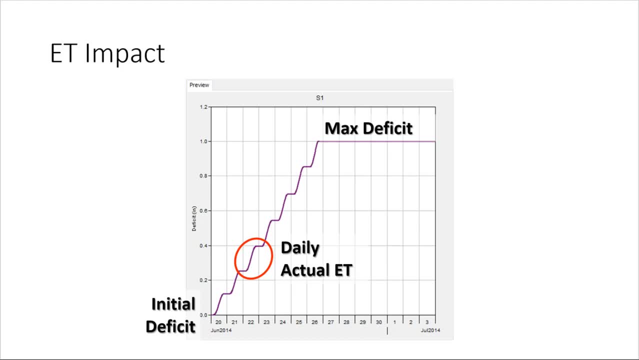 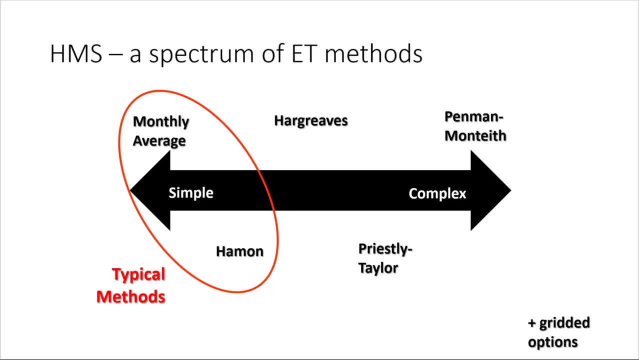 The initial and maximum deficit are controlled by the subbasin loss method. HMS includes a range of evapotranspiration methods. The simplest is to choose the monthly average value, which for some regions may be published data. The modeling requirements go up as you move towards the right. 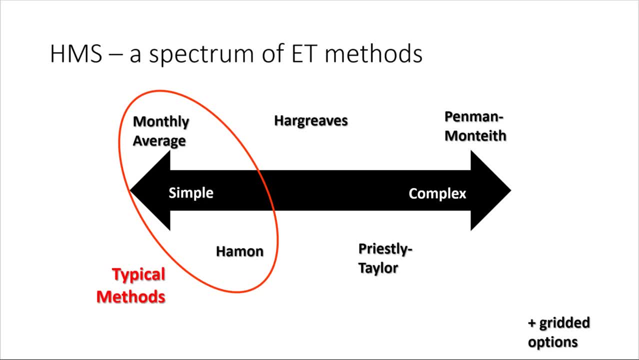 The Hammond method is a temperature-based PET method which approximates the energy balance using temperature data. The other methods begin to require radiation, wind speed and relative humidity data. In data-limited environments, the first two methods are usually adequate. Consider the role of ET in your model. 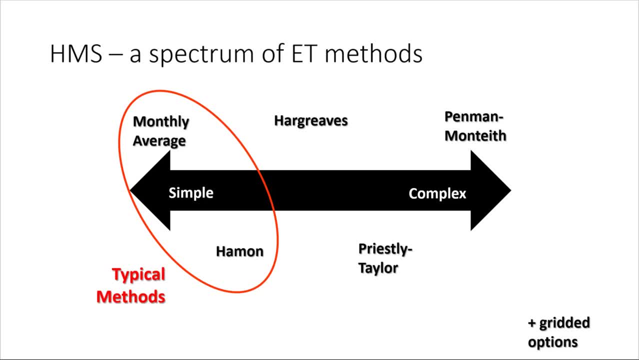 If you are most interested in large flood peaks, then spending a lot of time on additional details for ET may not make sense. Most of these methods have gridded counterpoints, but there are other parts as well where the input data is specified with grids instead of time series. 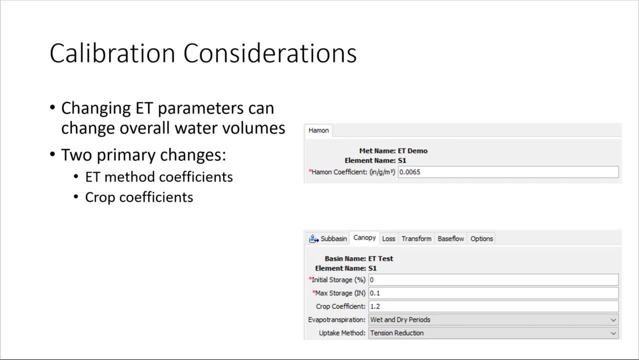 Only consider making adjustments to ET parameters if there is volume error that you suspect is attributable to a mismatch in the type of vegetation in play. In some locations, using a crop coefficient equal to 1 is not reasonable when the vegetation tends towards higher ET. 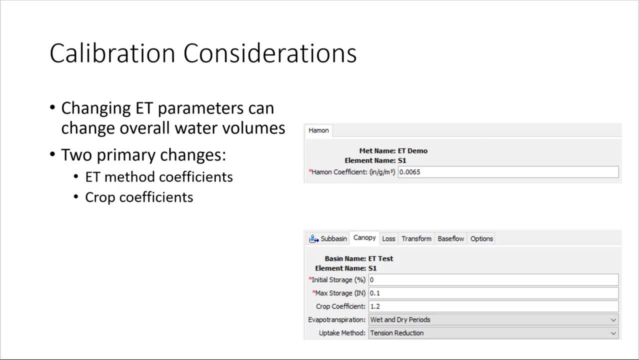 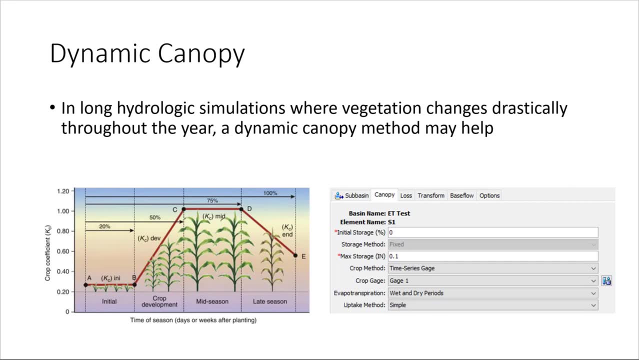 for example corn during the peak of its growth. You can also toggle between whether or not HMS will compute ET during periods when precipitation occurs. For long-term continuous hydrologic modeling, HMS is capable of simulating a dynamic canopy which varies the crop coefficient throughout the simulation. 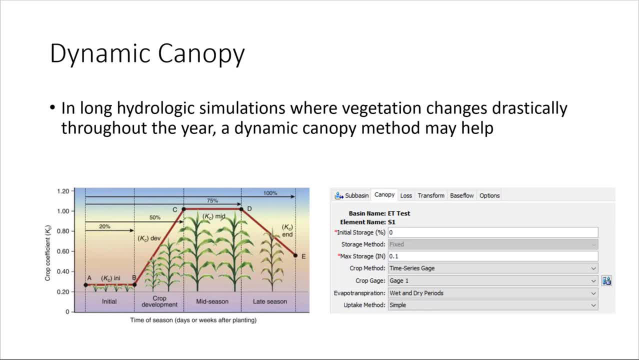 using a time series gauge or a grid set that you provide. I would only suggest using this approach in situations when modeling soil moisture deficits throughout the year can't be captured with a single crop coefficient. Here are the three key takeaways for evapotranspiration modeling in HMS.